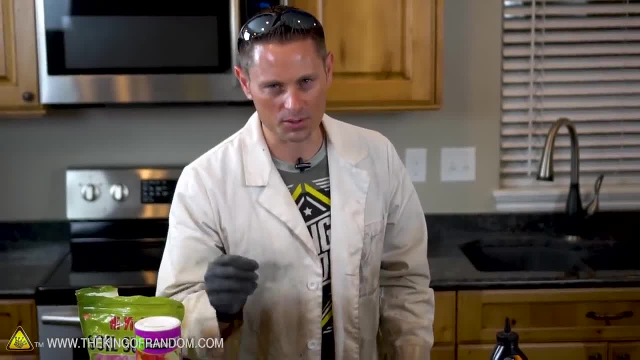 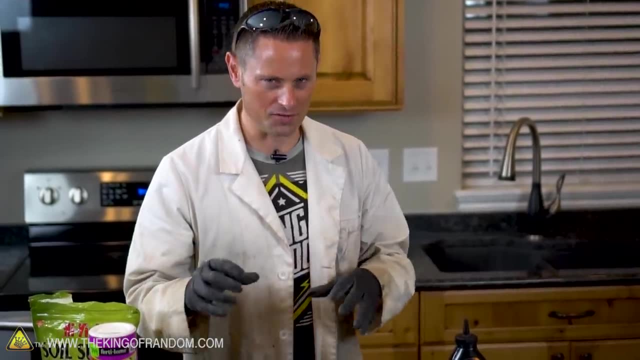 but if you mix them together in the right ratios, the results can be explosive. So now that we've gathered up all of our individual ingredients, the first step in making our black powder is to crush them all into very fine powder. It's very important we do this in separate containers, because we don't want those powders to mix together yet. 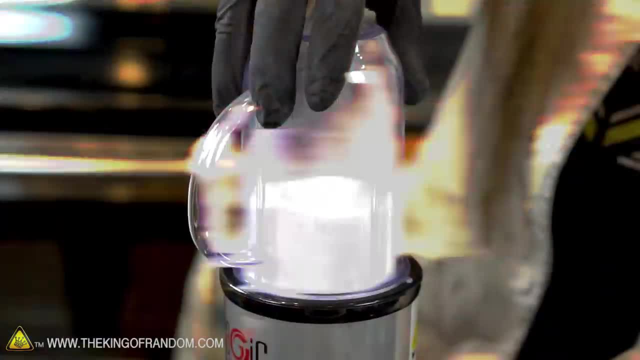 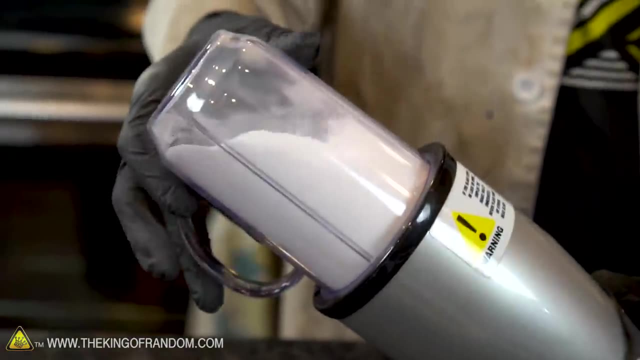 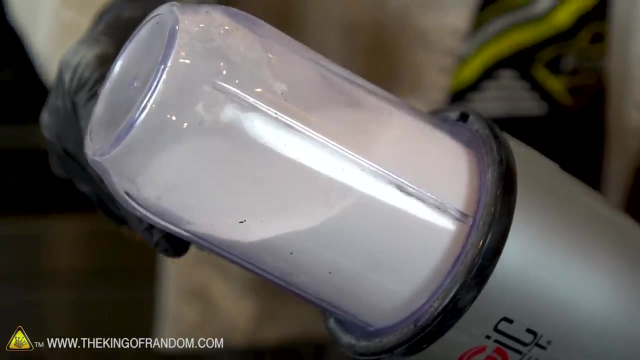 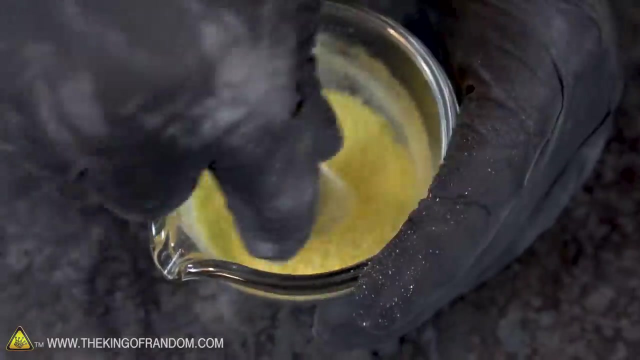 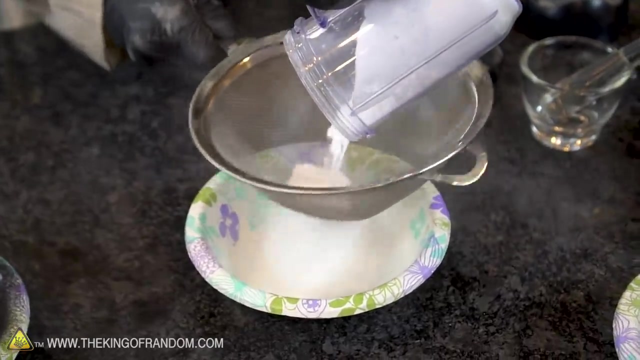 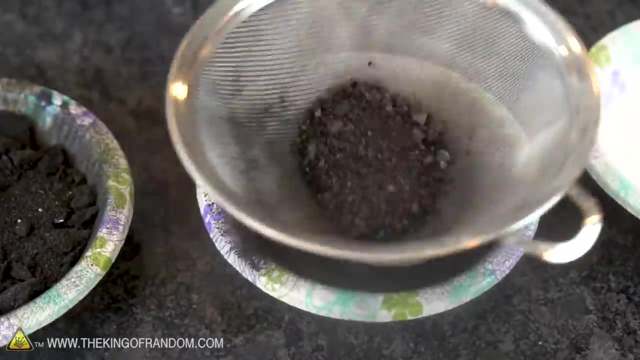 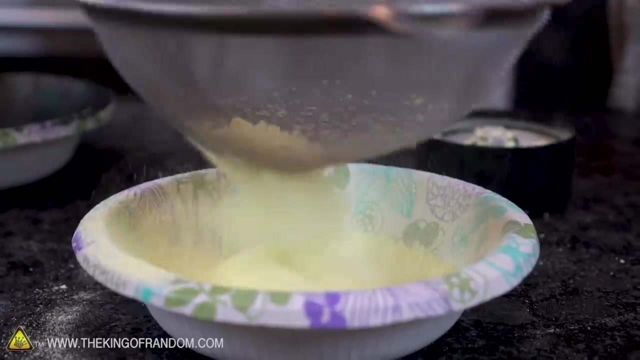 So let's go ahead and get busy crushing this stuff up. You can either get the powder out at once or you can crush it with the Charcoal paste. Beautiful, This is looking good. I'm getting excited. So update guys. I've just got all three of my powders finely floured and this is how I did it. I took out all of my powder and I crushed them all down with a lasci-mash through a sieve, which I'm gonna do that with a Shinse willst and a sieve. So, update guys, I've just got all three of my powders finely floured and this is how I did it. 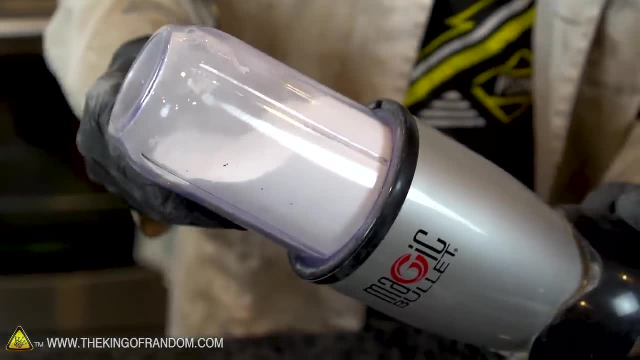 individual containers and a blender, and I blended it into a fine powder and then used a strainer to gently sift out only the finest particles. Now, in the case you don't have a blender, you could always do something like a mortar and pestle This. 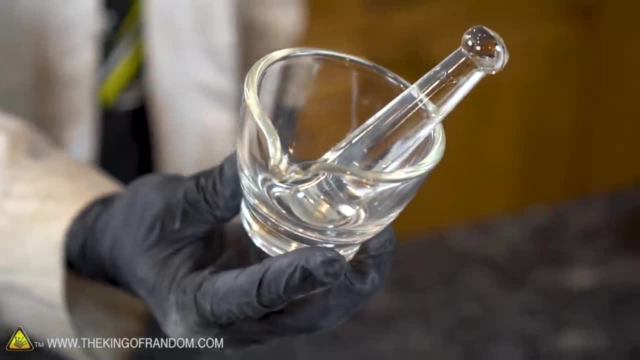 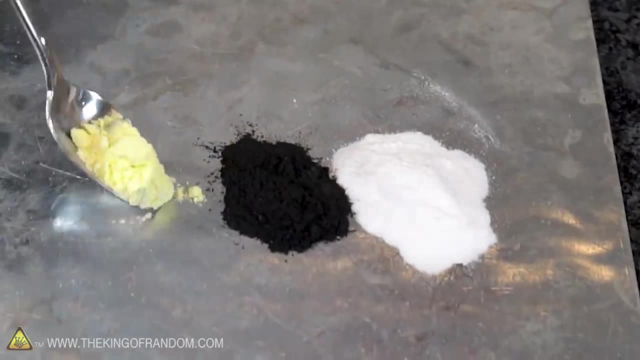 is basically a bowl with a stick that just crushes up the powder. In either case, it's still a really good idea to use a very fine strainer to filter out only the smallest particles. Now comes the fun part: we get to mix it all. 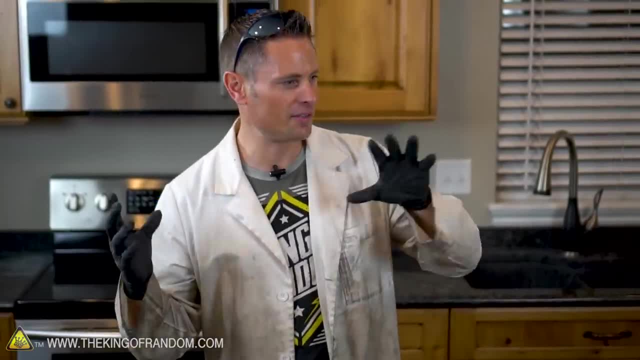 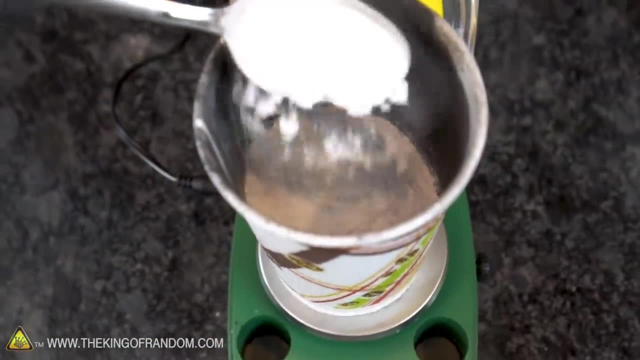 together. Now I'm gonna be using the traditional ratios that trace back thousands of years to when the Chinese first discovered this and used them in their fireworks. It's a very simple ratio of 75% potassium nitrate, 15% charcoal and 10% sulfur by weight. Now, potassium nitrate by nature is 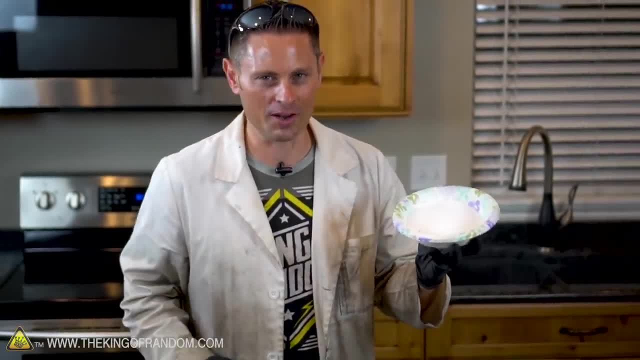 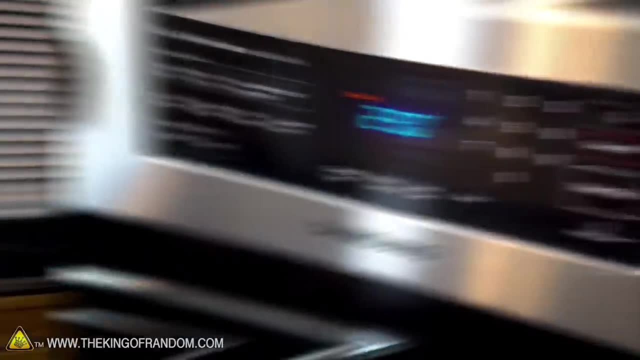 hygroscopic. it pulls moisture out of the air and that's not good for gunpowder. So before we mix these powders together, I'm just gonna bake this in the oven for about 25 minutes. Okay, so our potassium nitrate's been in the oven for 25 minutes, let's get it out. 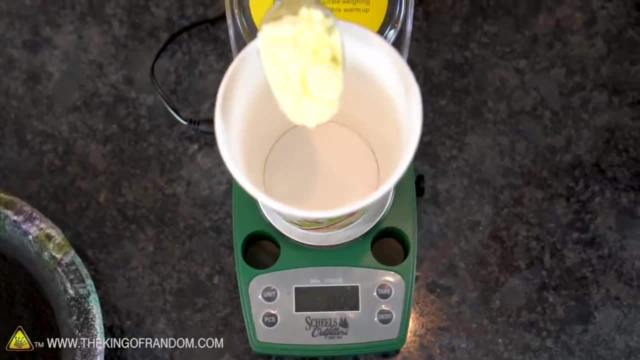 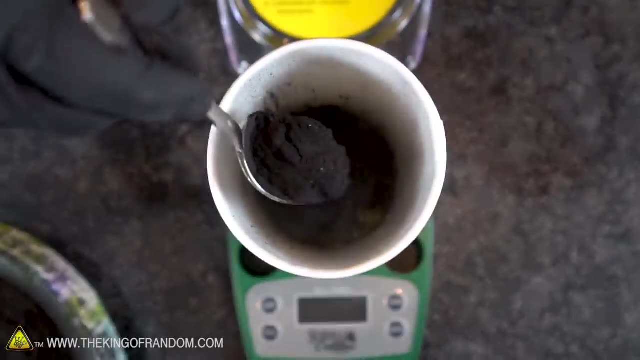 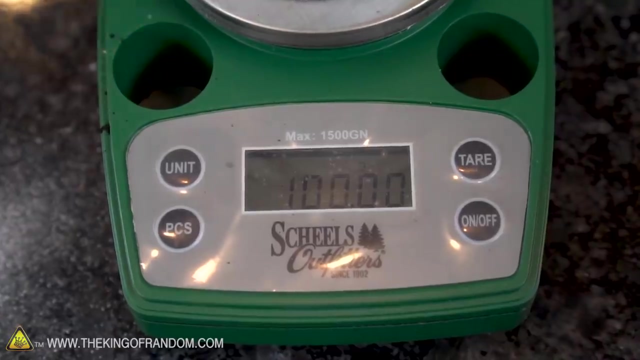 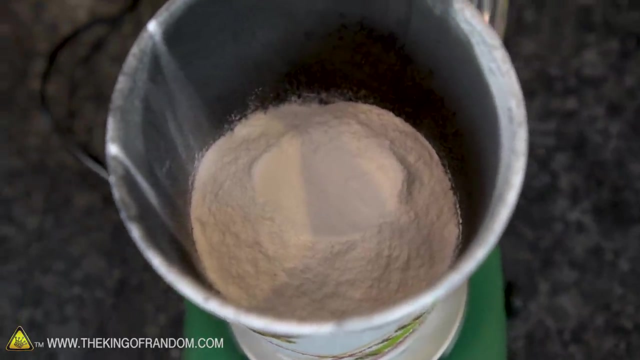 let it cool down and mix these three powders together. Now, to keep things nice and easy, I just mixed up a 100 gram batch. I used 10 grams of sulfur, 15 grams of charcoal, 75 grams of potassium nitrate. Now that we've, 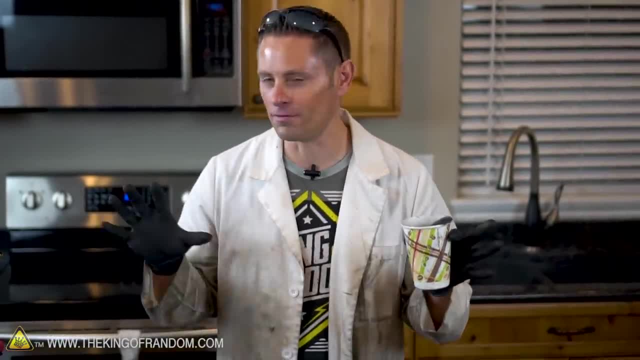 got these powders in contact. it's important to be very, very careful and do this in a fire safe area. Good idea to have a fire extinguisher nearby or, even better, to be outdoors in the open air. When we mix this, we don't want it to be. 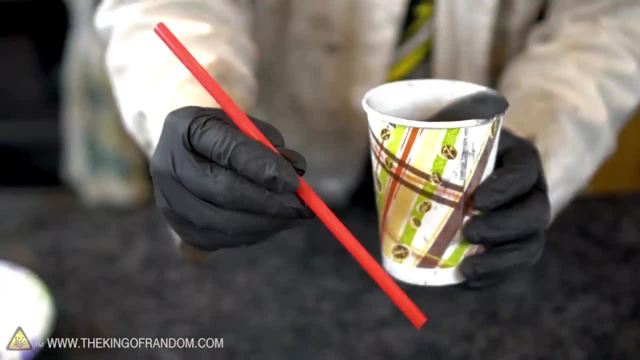 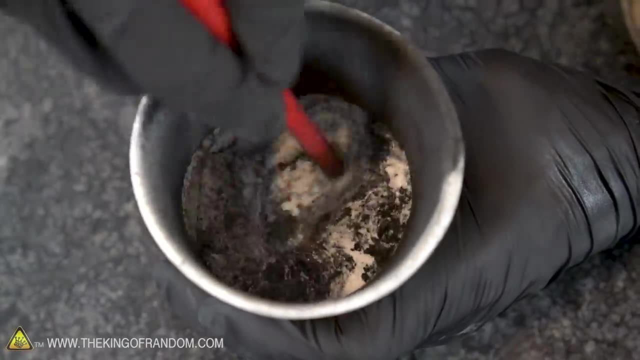 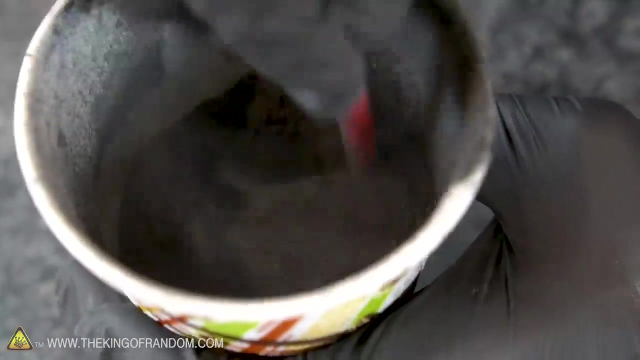 hot. we don't want to use metal because it's conductive. we want to use something like wood or plastic, The idea being that we just want to prevent any static electricity from being discharged into the mix. Our white powder has just become black Black powder. It's extremely light and 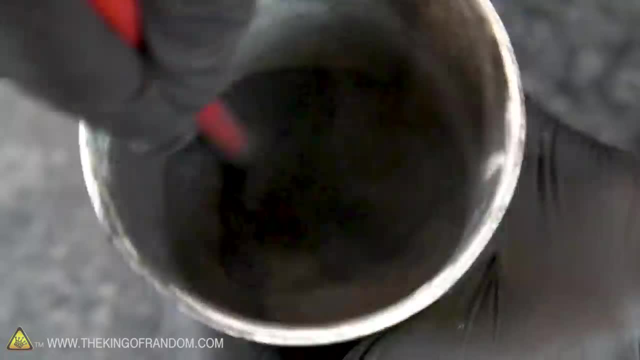 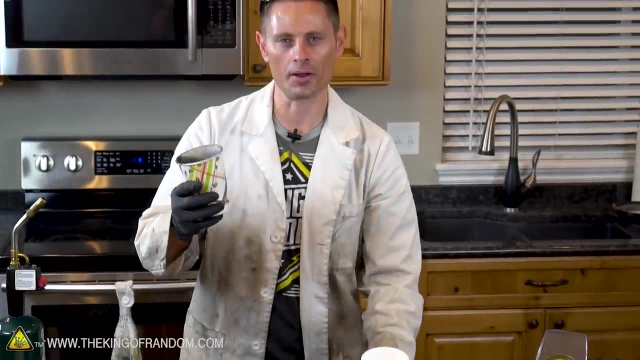 fluffy. that's very surprising, probably because of the charcoal. I wonder if I can blow bubbles in it. Not very well. Now, just to make sure this gets mixed up a little more thoroughly, I'm going to pour this into a bowl and I'm going to pour this. 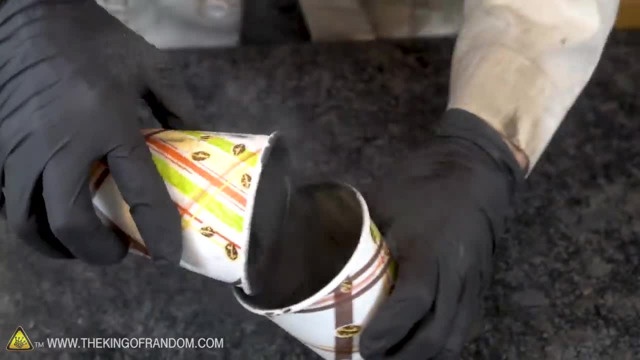 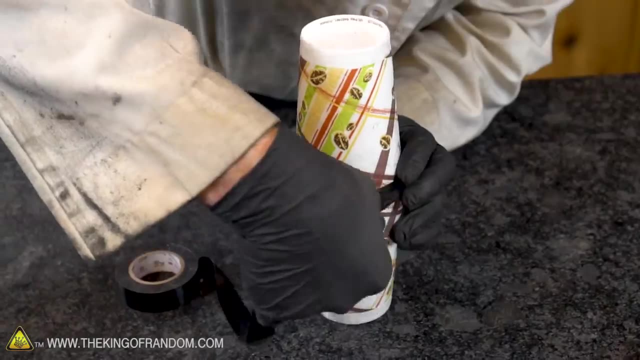 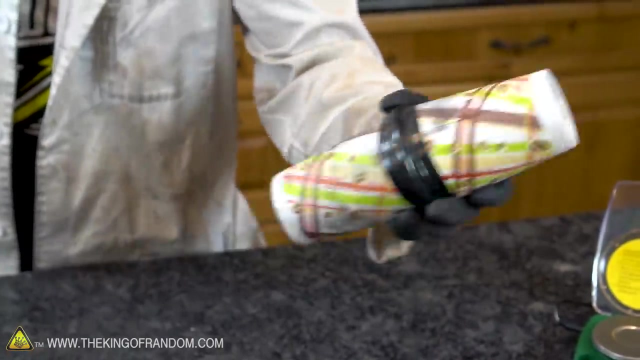 back and forth between two cups, Give it a shake, give it a stir, and just do my best to make sure these three materials are intimately combined. Keep away from sources of ignition. Boom And it goes off. So there we go. I've been shaking and 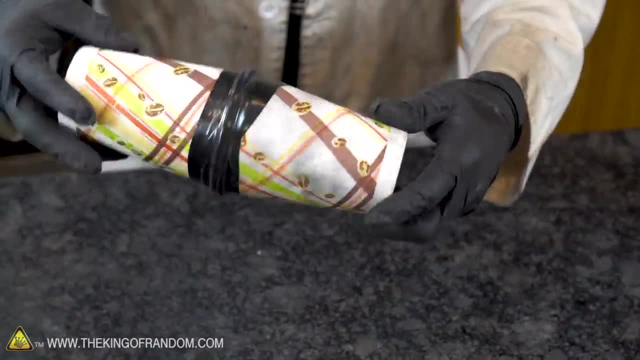 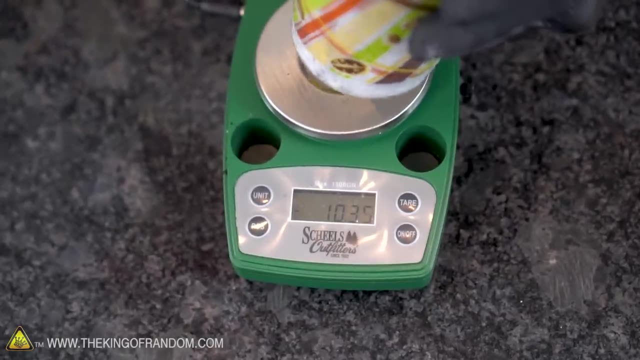 stirring this thing about as intimately as I can get it for the last two minutes. Hopefully by now it's thoroughly constituted. So let's pull out a small spoonful light, a match, and see if we can touch it off. All right, Weighing our composition, the verdict is 98.5.. So we lost about a gram. 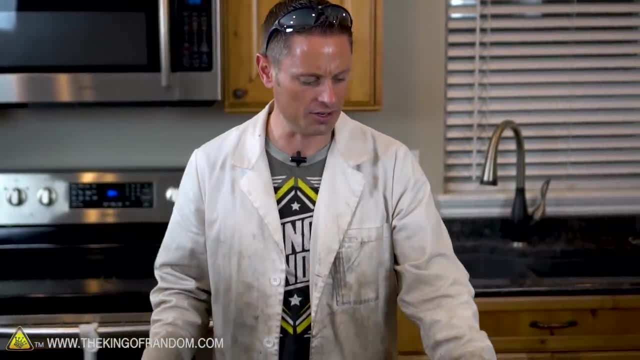 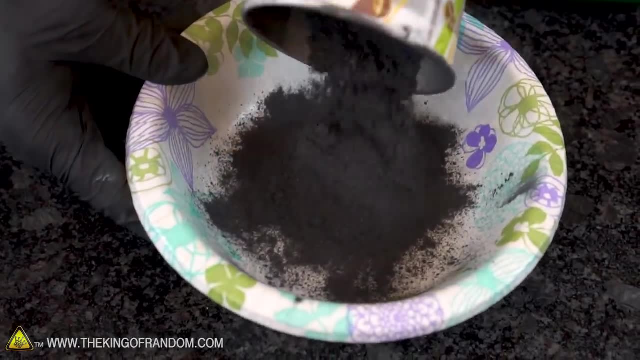 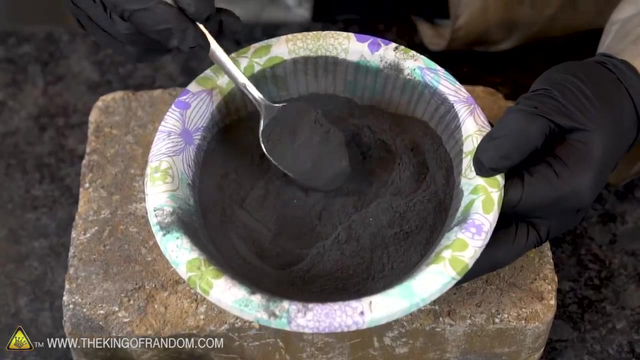 and a half in the process, But that's okay because we've still got a lot. In fact, 100 grams is probably too much. Right here, guys, is our homemade black powder. Looking good, Looking good, Beautiful. So I just realized I measured out a heaping tablespoon of this powder. 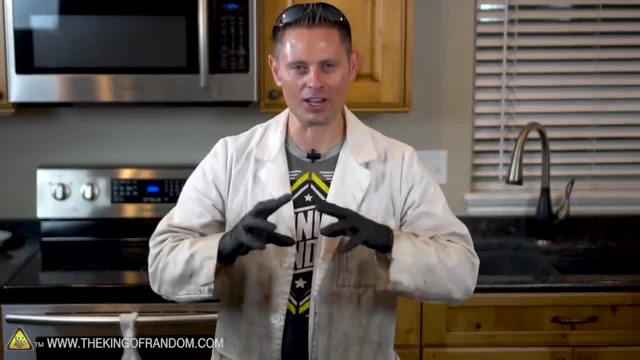 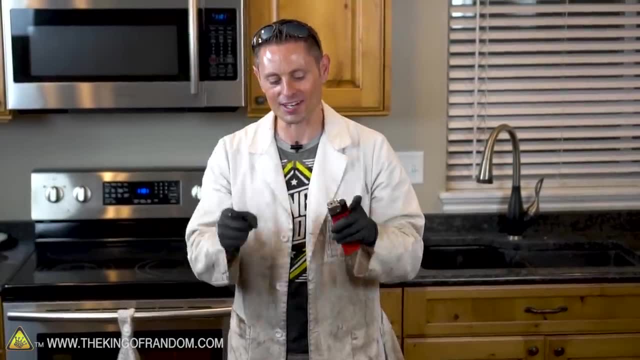 which is way too much, because if this were, then when it goes off it's going to make a huge cloud of black smoke. But that's something I'm totally willing to do for you. It's time to light it off, guys, and I'm a little bit nervous because this actually is quite a bit of. 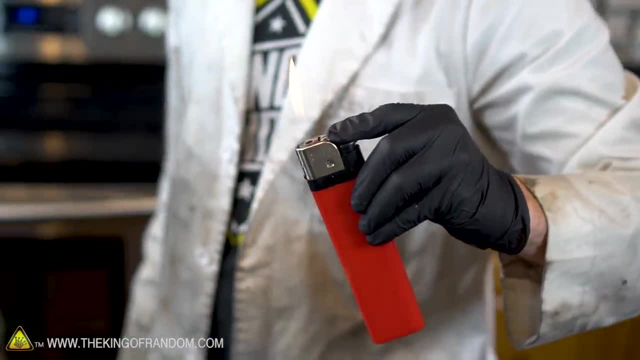 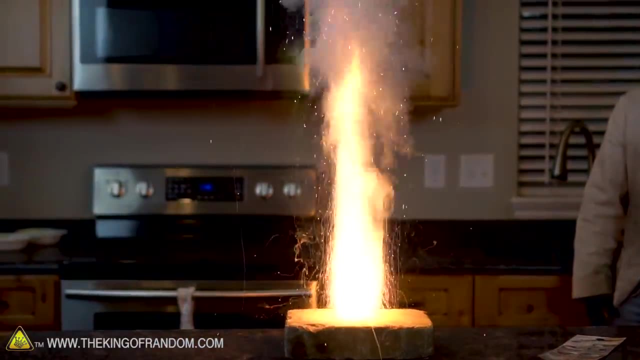 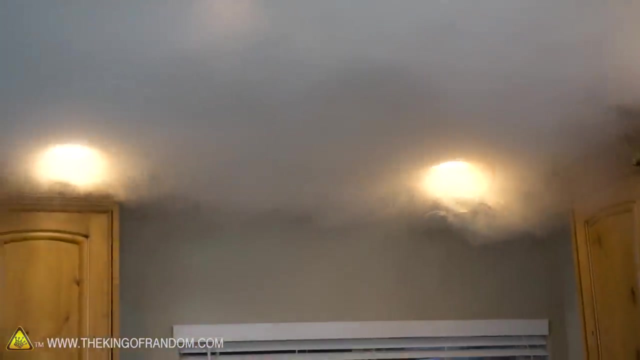 black powder. but let's do it Here we go, Nice, burn That put off quite a bit of smoke. That's what I would expect black smoke to do for me. I'm gonna take my fleeeek. I keep going, keep going. Each time I toss and one light your can for 10 seconds on the żeby, next time for another one Like this. That's something I'm. 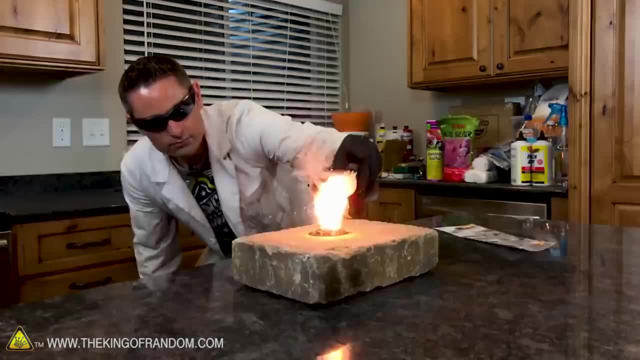 powder look like. I would say that was a success. so that worked and it pretty much worked the way I was hoping it would. it looked like kind of a slow burn, but that's only because it's in the open air if we cram this into something like: 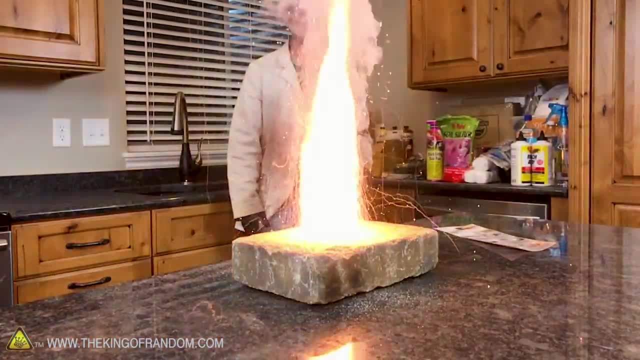 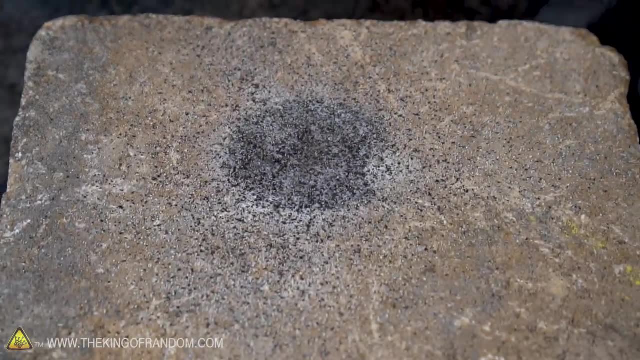 a firecracker it would go off with a bang. look at the residue here you just see a little bit of ash, but it looks like everything has burned completely. looks like our composition was just about perfect, very pleased. one more thing I want to try really quick is make a small line of this powder to make an 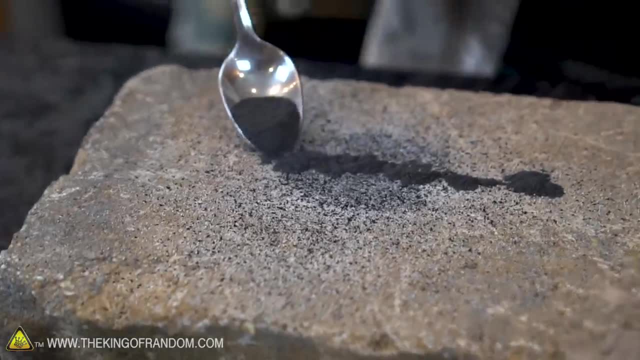 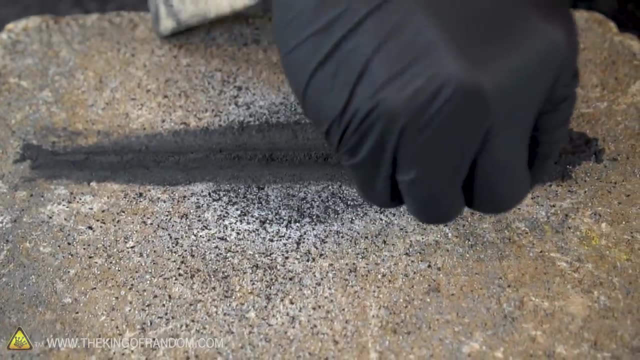 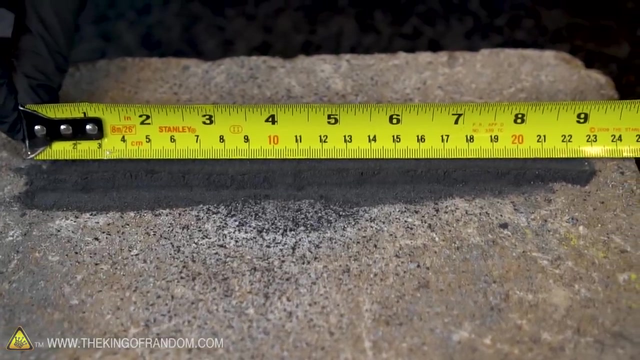 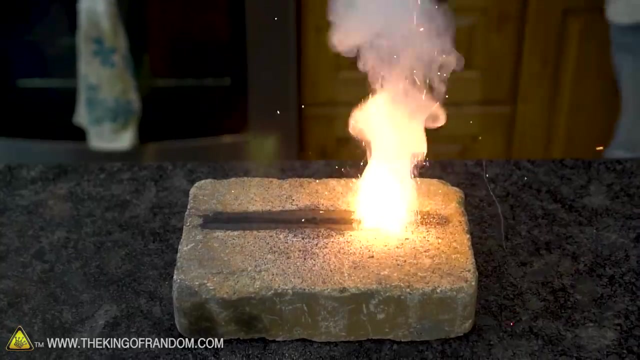 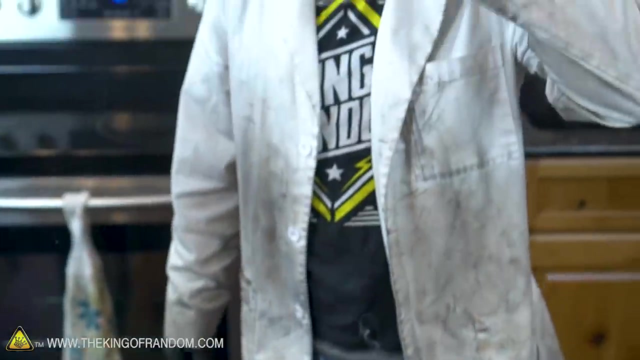 improvised fuse, beautiful, all right. test number two: I've laid out a nine-inch strip of powder to act as an improvised fuse so we can test the burn rate. here we go, sweet you. so a nice, very consistent, slow and steady burn, that's exactly what we want. 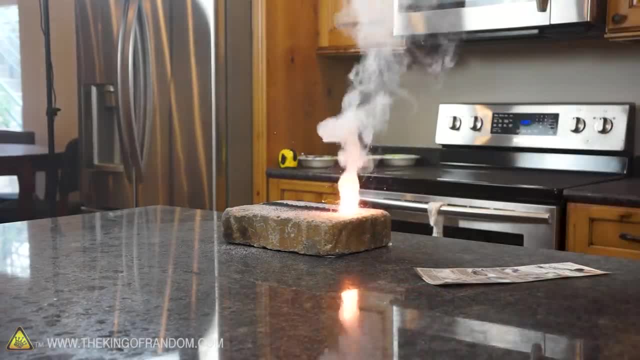 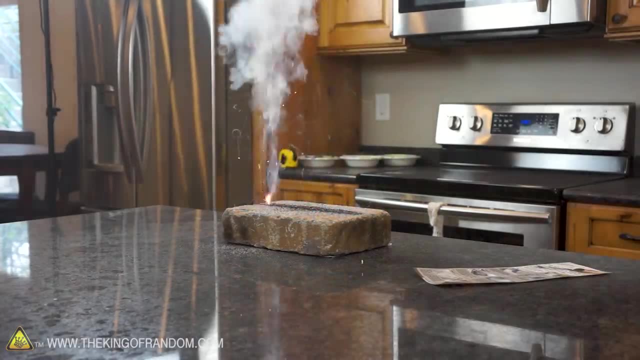 to see now. this burns relatively slowly because it's in the open air. if it were in a confined container, the burn rate would increase exponentially and probably make the container explode. so, guys, our black powder works. it looks great, it burns really well. so let's do a quick summary of how we got to this. 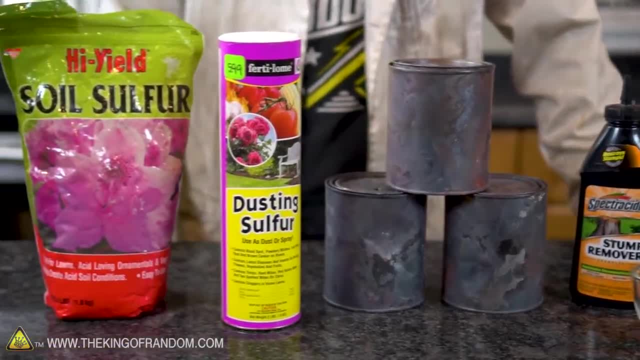 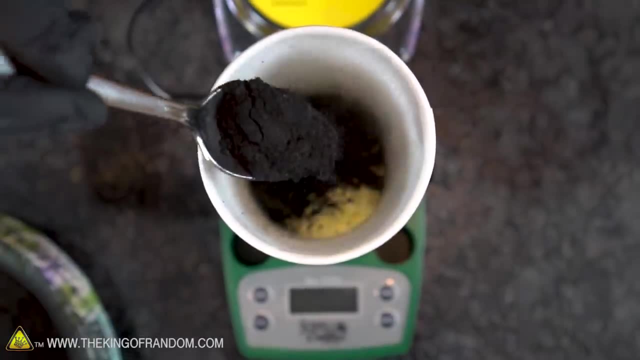 point. we start off with three different materials: potassium nitrate, charcoal and sulfur. we ground those materials into a fine powder, then used a strainer to sift off the finest materials and mix them together in a ratio of 75 percent, 15 percent and 10 percent respectively. we used a plastic straw to stir them. 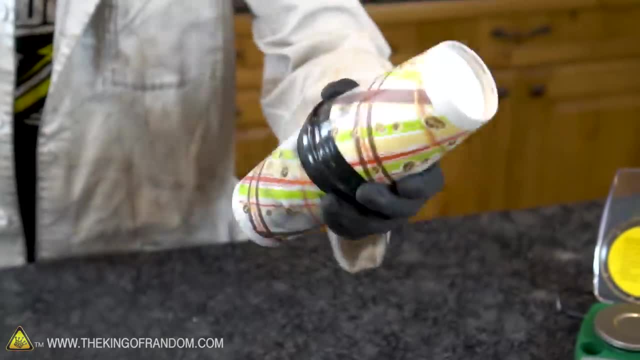 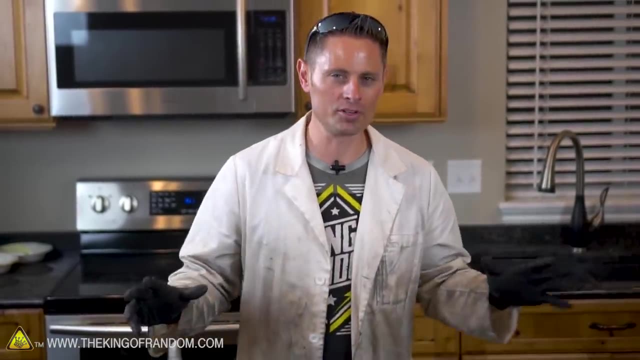 together, then tape two cups together to shake it for about two minutes, which resulted in this fine dark gray composition we call black powder. and black powder doesn't necessarily have to mean gunpowder. there are far more uses for it than that. it can be used for making fuses, rockets and fireworks, and